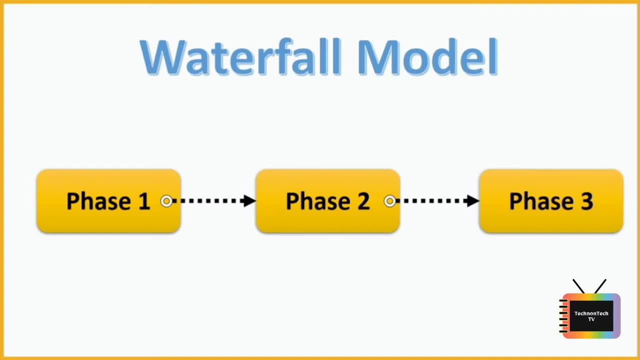 each phase requires deliverable from the previous stage. So requirements are moved to the design phase, design moved to development and code made during the development phase is moved to the testing. So that is why we call it as a waterfall model or linear sequential model, First complete. 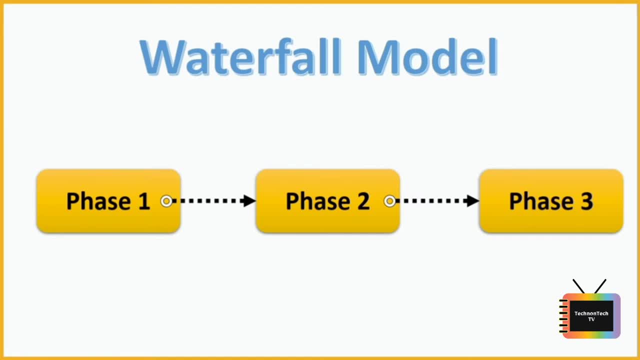 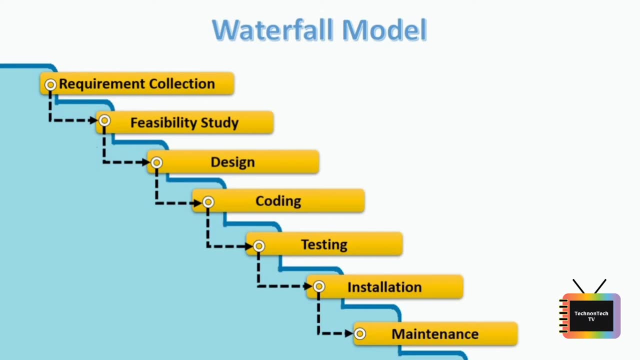 the first stage. So without completing the first stage you cannot move to the second stage. So this is the basic stage of waterfall model. So if you are using waterfall model for your project, then these 7 stages will be added and removed according to your project. So this is. 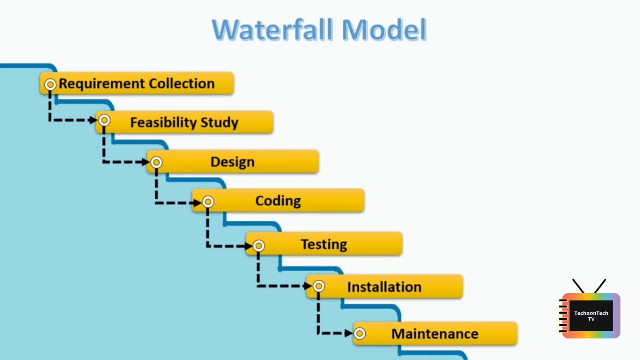 the basic stages. So if we look according to the books, then these are the basic stages, But if we are developing any software in real world, then different stages will be added according to the project requirement. The first stage of the waterfall model is requirement collection, where 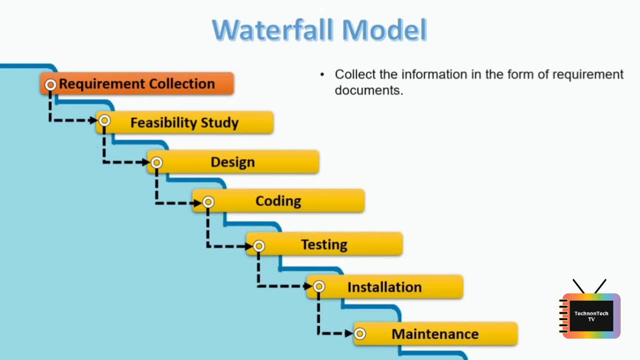 a business analyst will collect all the information and business need of the customer in the form of requirement documents. So in this stage, the requirement is collected with the help of SRS, CRS, BRS. So the business analyst will collect all the information and business need of the. 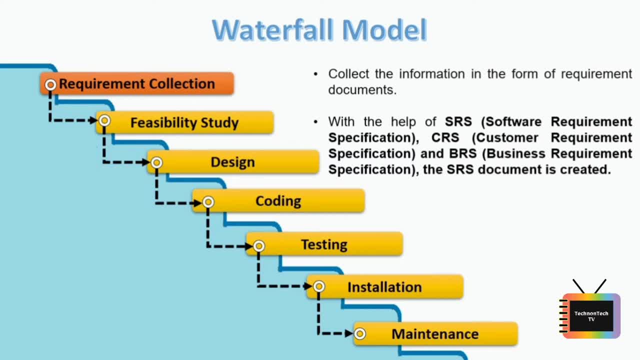 customer and he creates a final SRS document, And the document is collected by the business analyst. So the document should be clear and easy to understand and all the requirements are properly listed. The second stage of the waterfall model is a feasibility study. It is based on the 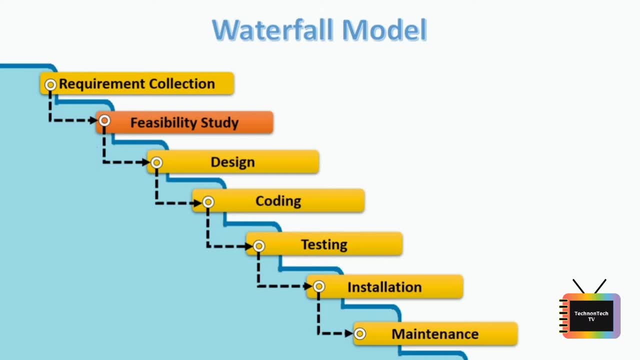 requirements where a set of high level people like business analysts, HR architecture, analyze whether the project is doable or not doable. So in the first stage all the requirements are gathered, but in the second stage the feasibility of the project will be checked. that the project 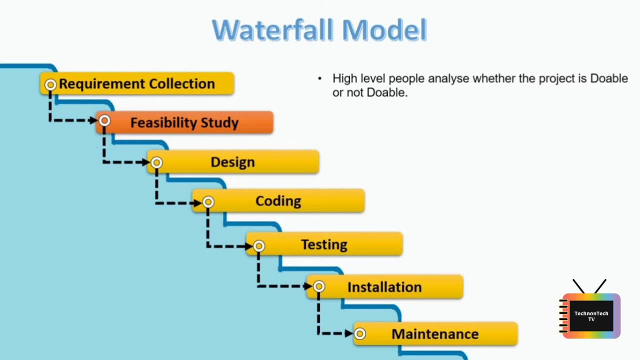 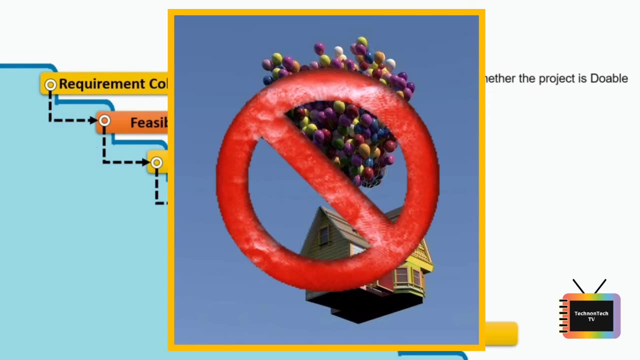 can be developed or not. So, for example, the project is that we have to make a house in the cloud, just like we saw it in the up movie. So this project is doable or not. Of course not right. So this feasibility, 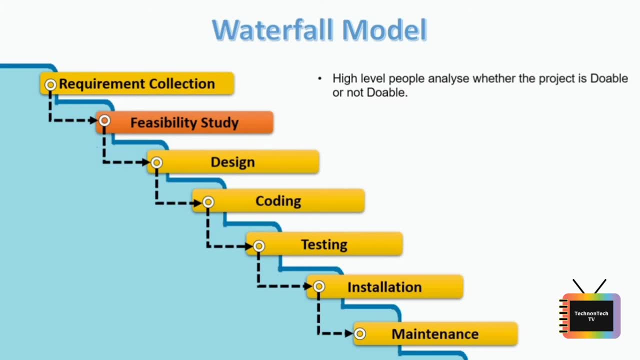 stage is just to analyze whether the project is doable or not doable. So an organization needs to have the different aspects to develop the project. First is economic: Can organization complete the application within given the budget or not? Second is operation feasibility: 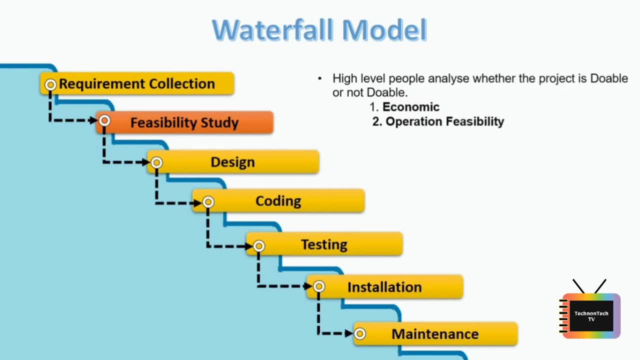 Can organization creates the operations which are expected by the customer? Third is technical. Here need to check whether the current computer system can support the software or not. Last is schedule. The project can be completed within the given schedule or not? So like that we have to check. 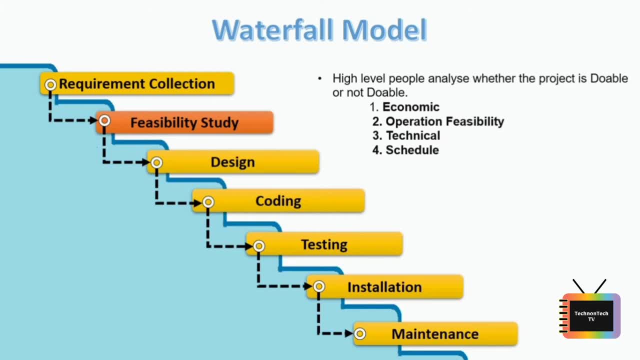 different aspects before going to design phase. Once the feasibility study is done, we move to the design phase. It basically defines the architecture of the project. So we have to design the architecture of the project. The designing phase specifies the essential tools required for the project, such as programming language like java, dotnet, php database like 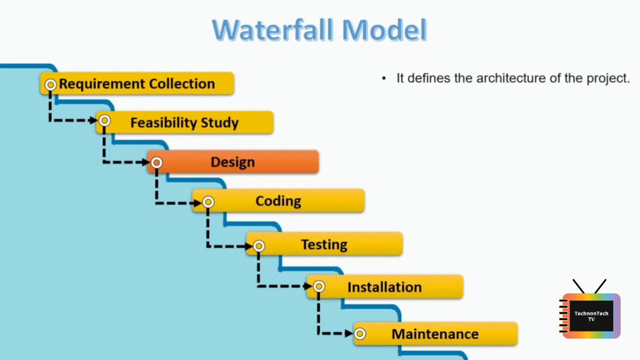 oracle, mysql and a combination of hardware and the software. After that, designers prepare a blueprint of an application which is divided into two parts: high-level design and low-level design. So in high-level design, designer will focus on making the model, So the design of that project. 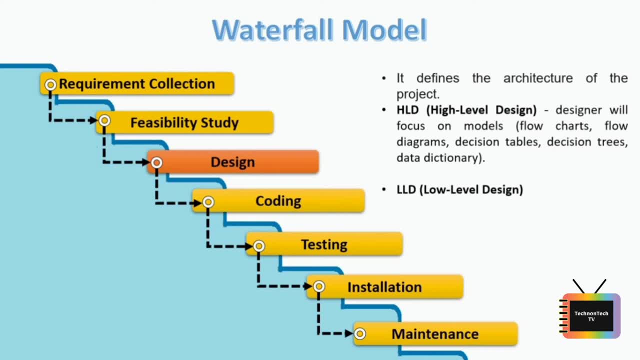 will be created through flow charts, flow diagram, decision tables, data dictionary, through right And in low-level design, designer will focus on components like UI design, So designer will create user interface. So, after the completion of requirements and designing phase, my requirement: 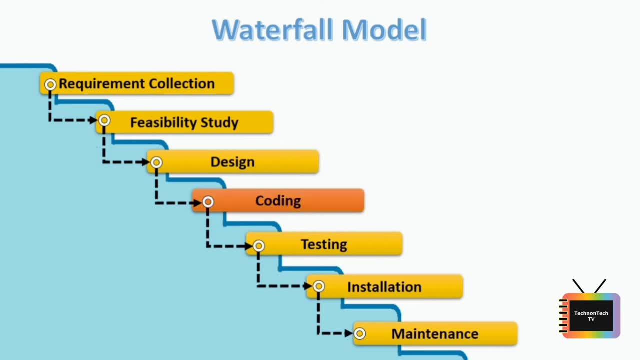 is clear. design is ready. Now the next phase is to develop a software system. So the developer starts writing code according to their programming knowledge and using the particular program language, like java, python, c++, c-sharp, etc. 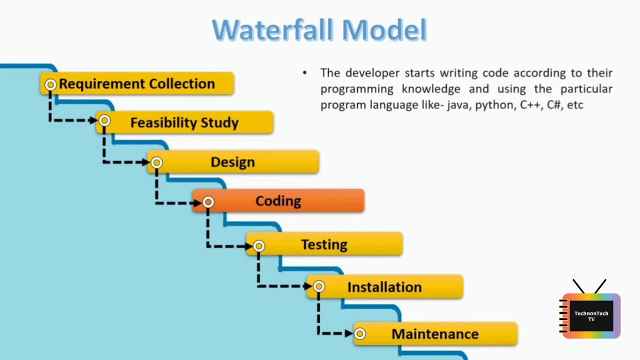 The front-end developers develop easy and attractive GUI and necessary interfaces to interact with back-end operation, And back-end developers do back-end coding according to the required operation. So once the developer completes the coding phase, the application is handed over to the test engineers, where they start checking the functionality of an application. according to the customer need or requirement. Basically, tester will test whether the system which is developed functions properly according to the customer need or not. So during the testing process, a test engineer may encounter some bugs or defects in the software which are not working as per the customer requirement. 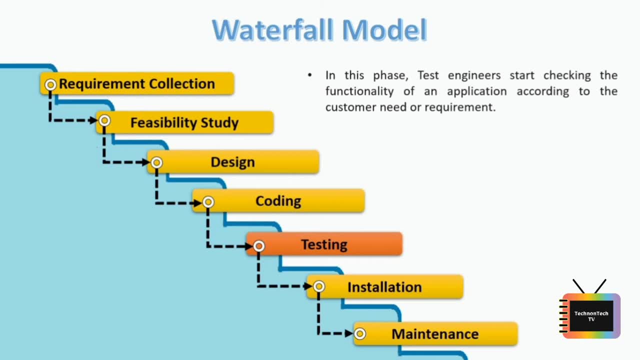 So, in case if the testing team gets any defect or issues, so what they will do is they send a bug to the development team with proper explanation and after that developer needs to check whether the bug is valid or not. if the bug is valid, then the developer will fix it and 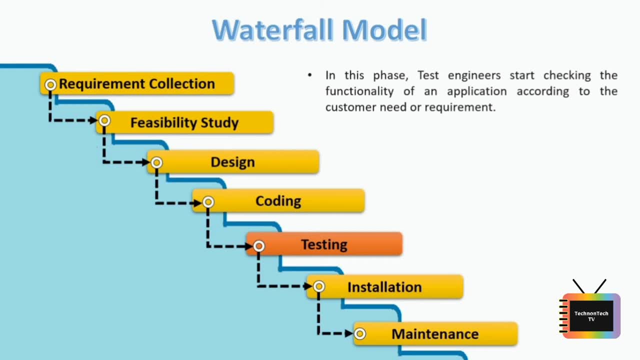 replace it with the new one, then it needs to be retested by the tester to check whether the bugs is fixed or not. but waterfall model ka sabse big drawback ye hai ke agar humne ek phase complete kar liya hai, then we cannot move back to the previous stage. so because of this there are high 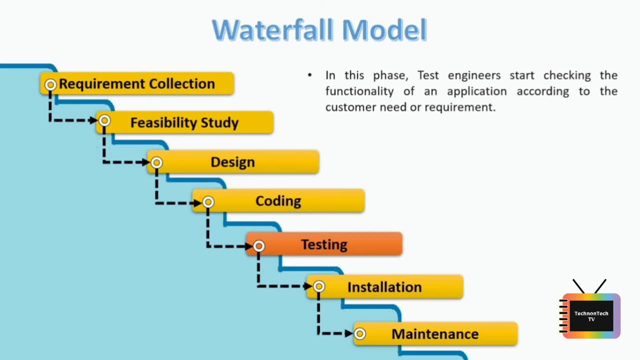 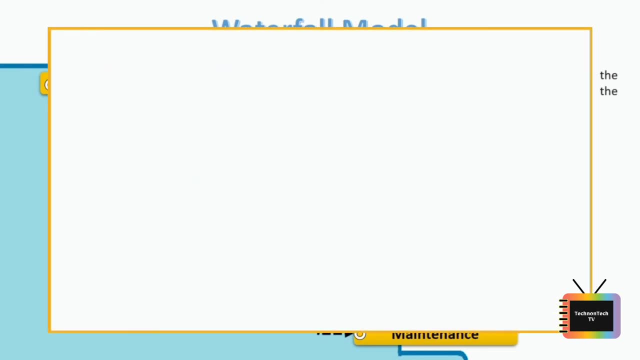 chances of risk. so developer ne toh develop kar diya aur hume defect pata chal raha testing stage pe. ya maintenance stage pe toh cost will increase. for example, ek company hai, ABC usne, apna project ke development ka contract diya hai XYZ company ko, aur testing ka contract diya hai PQRS company. 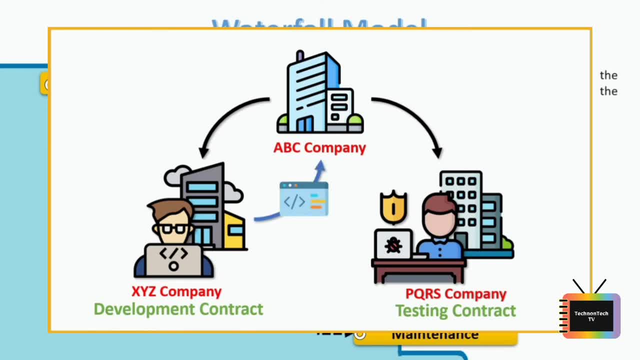 ko ok XYZ company ne apna development ka kaam kar kare de diya hai kya labour vadia hai, and ABC company has also paid it. and now ABC is handing over the project to PQRS company for testing and in the testing phase we are getting to know that there are a lot of issues. 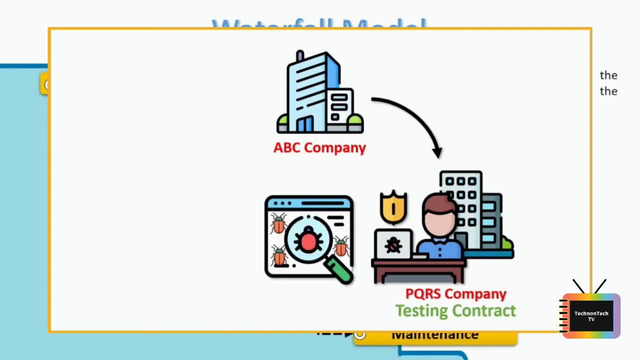 so again ABC company will have to hire some other company for development or for support. so here cost will increase. now the other company, let's say MNO, MNO company, will start all the phases from the starting, because MNO doesn't know the requirements. so time will increase and cost will also increase. 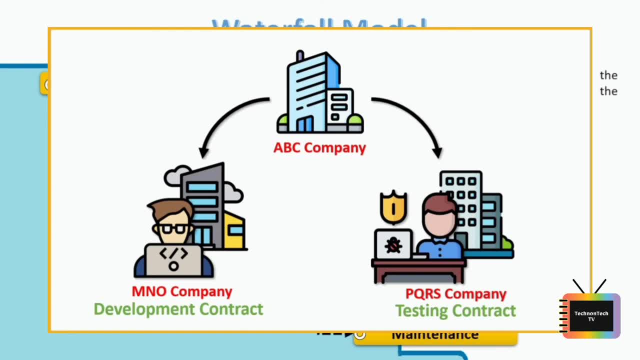 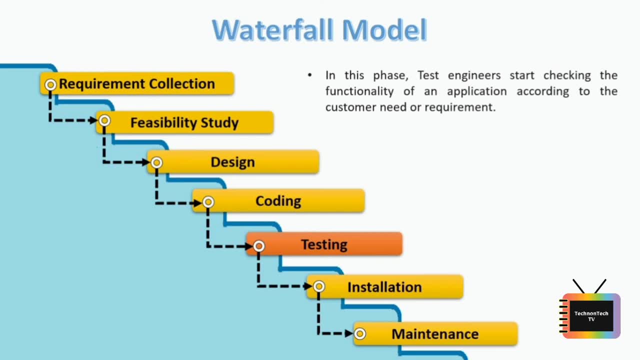 so this is the major drawback of waterfall model. so in waterfall model we cannot go back to the previous stage. so in waterfall the water always falls in the forward direction, it doesn't go in the reverse direction. so we have to follow the similar concept in this waterfall model. 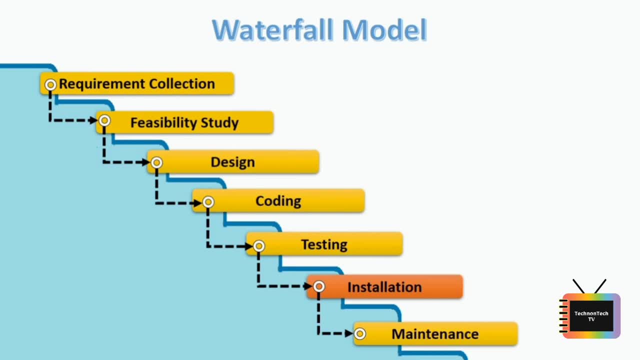 next is installation phase, so the process will continue until the application is bug free, stable and works according to the customer need. after that, the stable application is installed into the customer's environment for customer use and the last and long lasting phase of the waterfall model is the maintenance phase. 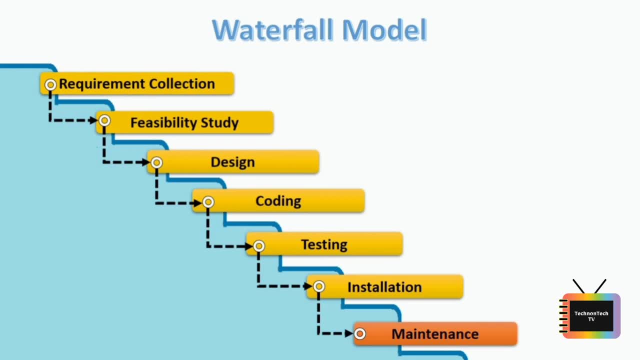 this process will continue until the application comes to an end. when a customer starts using the software, then they may have some issues, and they may have some issues which needs to be in detail tested and fixed. so maintenance phase also includes changes in software and hardware to maintain its operational effectiveness and improve its performance. 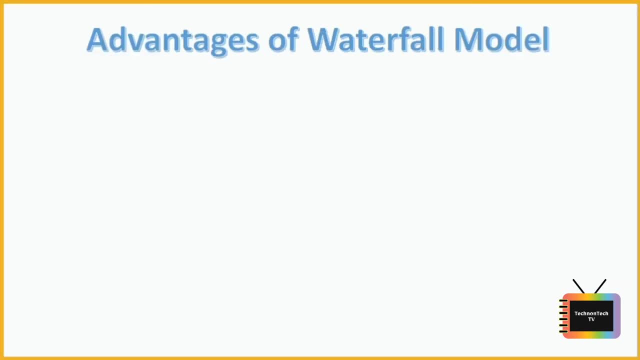 now let's see important benefits of the waterfall model. so waterfall model is very basic and simple model and we can use waterfall model only when the requirements are properly documented and clear. if the requirements are not clear, then we can use the waterfall model only when the requirements are properly documented and clear. 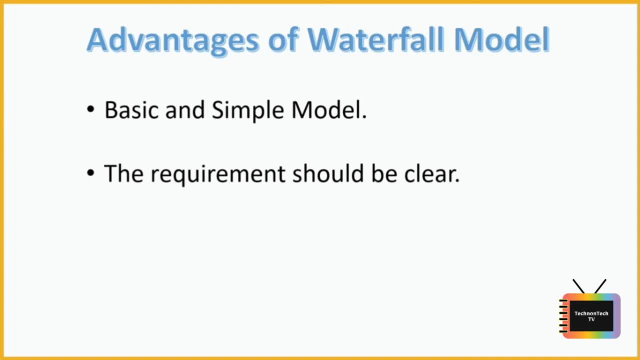 if the requirements are not clear, then the project needs to finish και we must leave it to the development phase. and if there are some issues, then again issues will arise. after that we'll go to the testing and maintenance phase. after knowing changes in software, then we cannot move to the development phase, right? 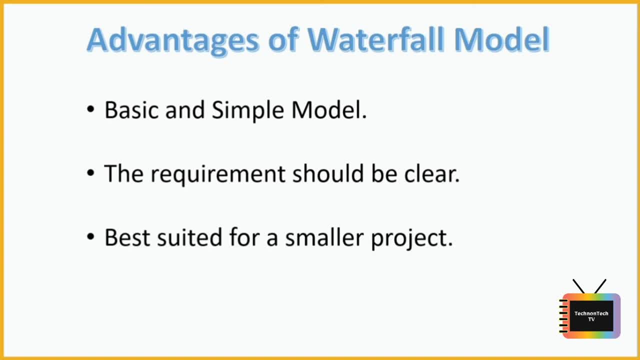 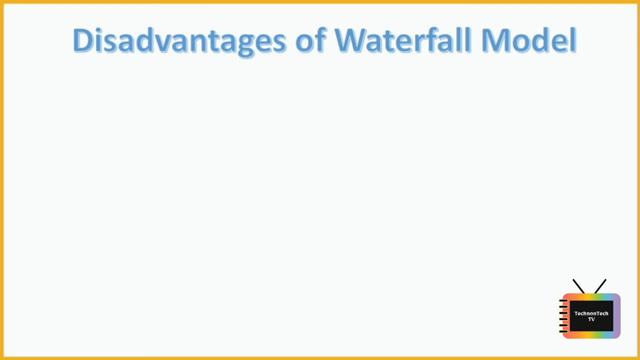 so requirements should be clear and this is best suited for smaller project where requirements are well understood. this model is not good for large and complex projects. next is disadvantages of waterfall model. so first one is no parallel deliverable. so main drawback is that we cannot parallelly work on two or more stages. 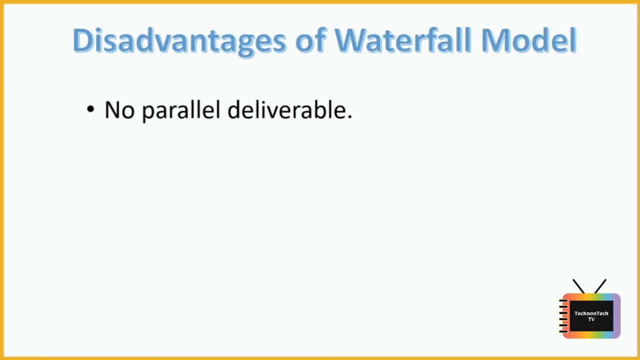 we have to first complete the first stage. then only we can move to the second stage. next is requirement changes not allowed. once we move from requirement phase to design phase, then after that we cannot again change the requirement. that is why if you are using the waterfall model, which is nowadays is very rare, then the requirement should be very clear. 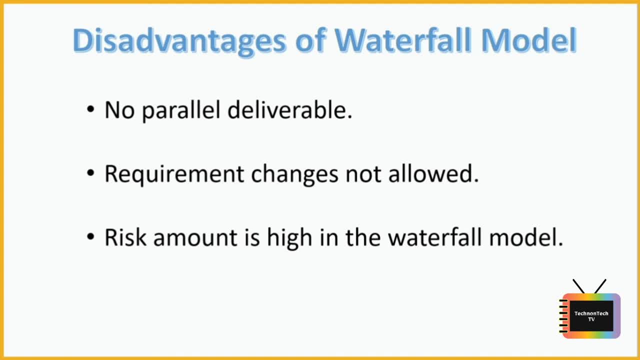 next is: risk amount is high in the waterfall model. so i told you earlier right about abc company. so if risk will increase, cost will automatically increase. so that's it for this video. if you have any doubt, comment us below, and if you found some value in this video, then make sure to subscribe to the channel and give me a thumbs up. 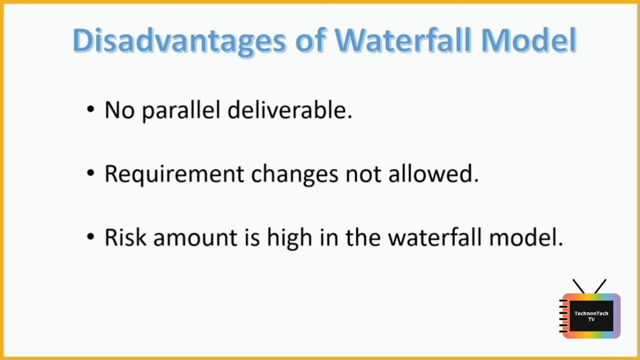 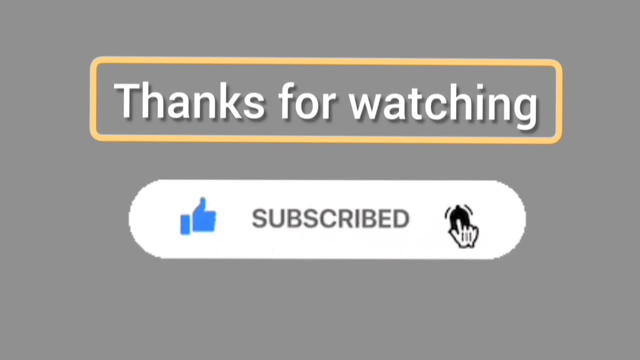 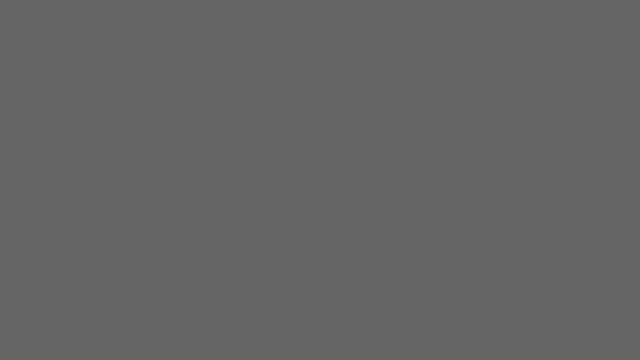 and do share this video with your friends to spread the knowledge and stay tuned for more videos. thanks for watching.